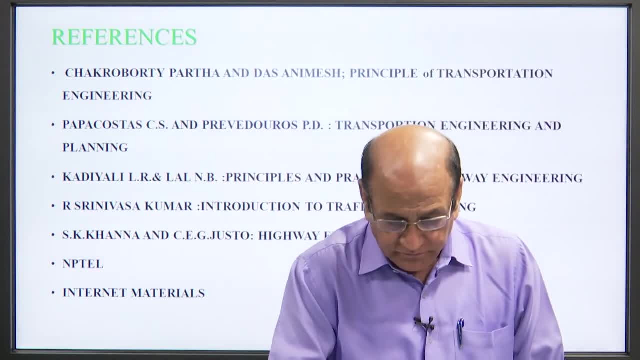 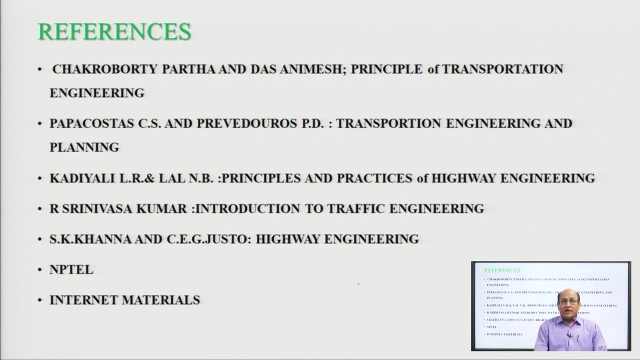 management. References we have taken: Chakravarti, Partha and Das Animesh, Principal of Transportation Engineering, Papacosta and Pravedendas, Transportation Engineering and Planning, Kadiyali and Lal, Principal and Practices of Highway Engineering or Srinivas Kumar, Introduction to Traffic. 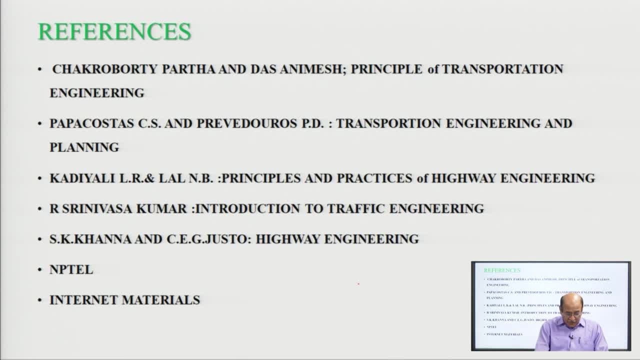 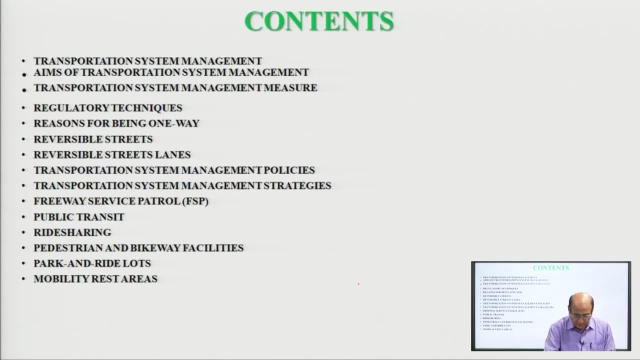 Engineering, S K Khanna and Justo Highway Engineering, and some material have been taken from DAPTEL and Internet Content. today we will cover transportation system management. aim of transportation system management. transportation system management measures- regulatory techniques, reason for. 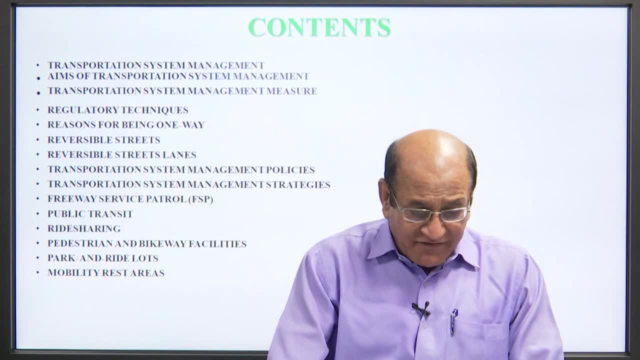 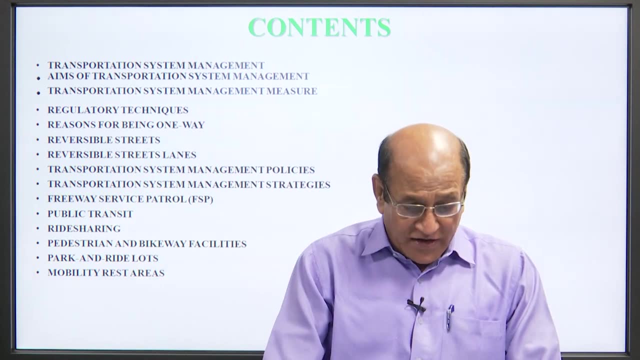 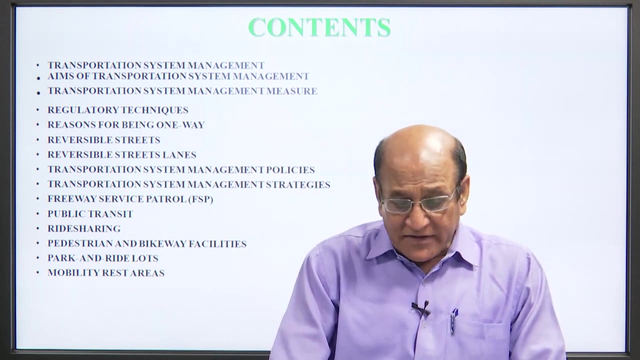 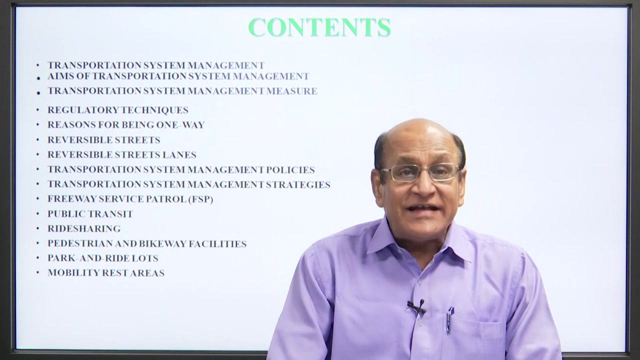 being one way: reversible street, reversible lane. transportation system management policies. transportation system management policies. Transportation system management strategy. Free way service, petrol, public transit, ride sharing, pedestrian and bike way facilities, park and ride lots, mobility rest areas. 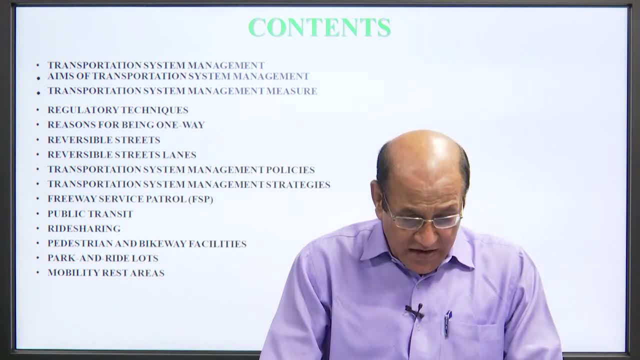 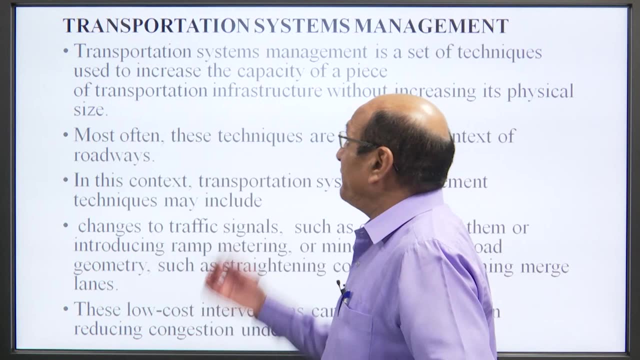 loading and gassing. All this together, consider that most potential application related to transportation system management of roads or streets, tunnels towards of exits to kannada, community method of transportation. We will take up one by one. First of all, transportation system management. What is? 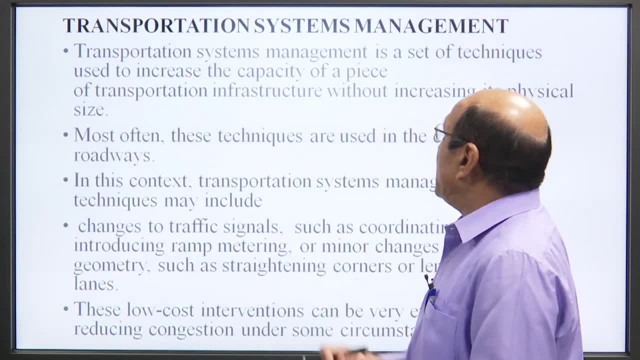 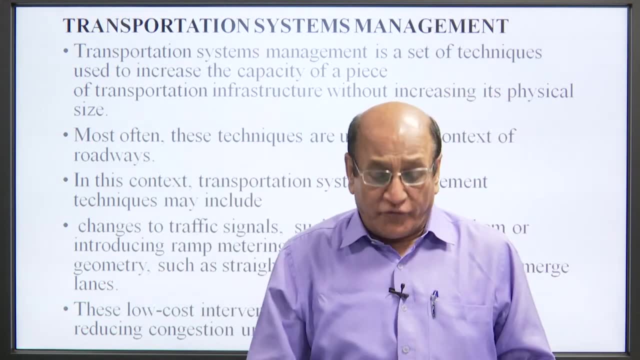 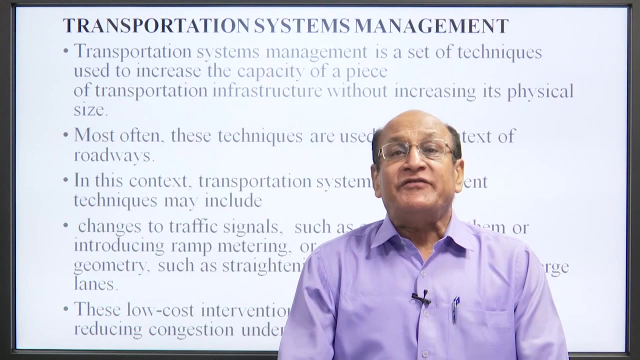 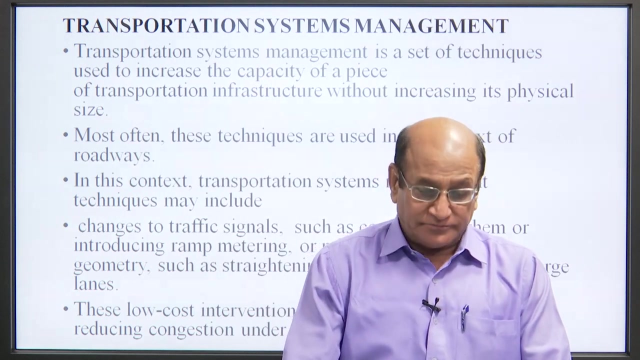 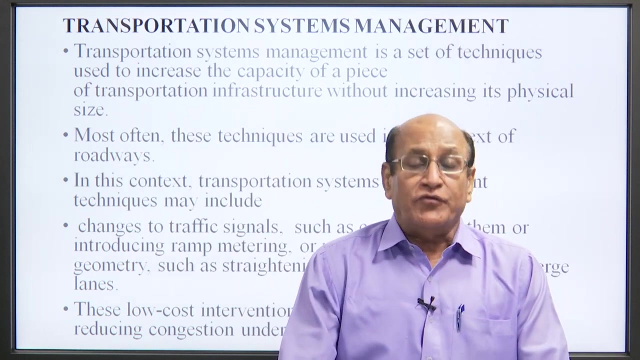 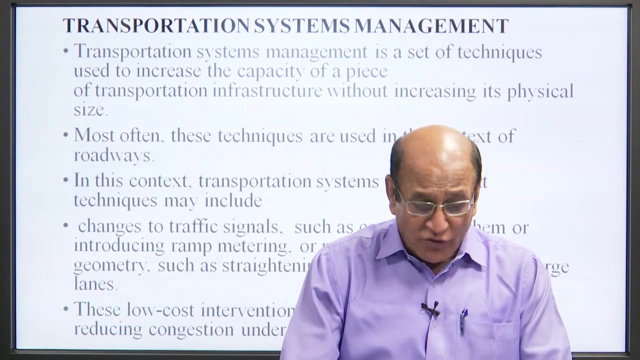 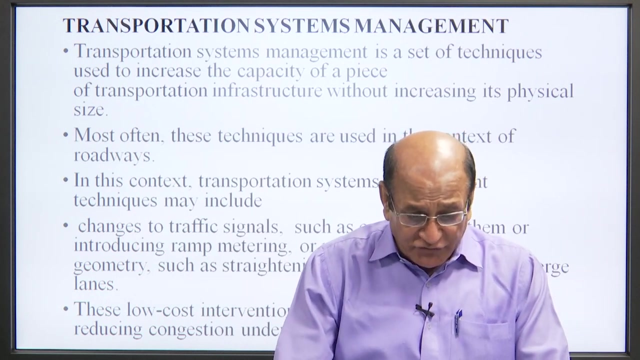 transportation system management. Transportation system management is a set of technique used to increase the capacity of a piece of transportation infrastructure without increasing its physical size. Most often, these techniques are used in context of roadways. In this context, transportation system management technique may include change to traffic signal, such as coordinating them or introducing ramp metering. 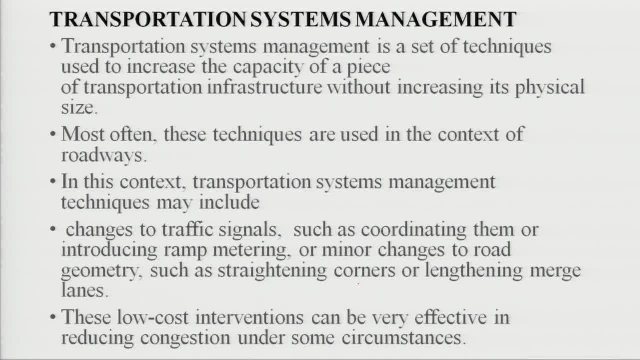 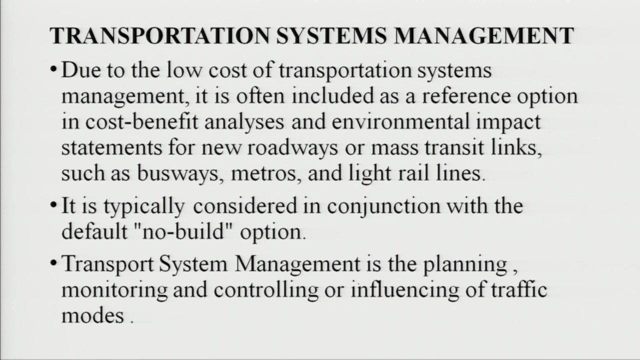 or minor changes to road geometry, such as a strengthening corner or lengthening merge lane. These two cost intervention can be very effective. So transportation system management can be used to increase the capacity of a piece of transportation infrastructure, crying of the transportation structure. In addition, transportation system management can be used to beer as a reference option. 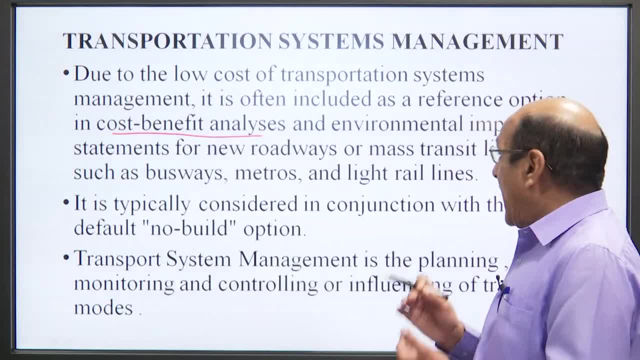 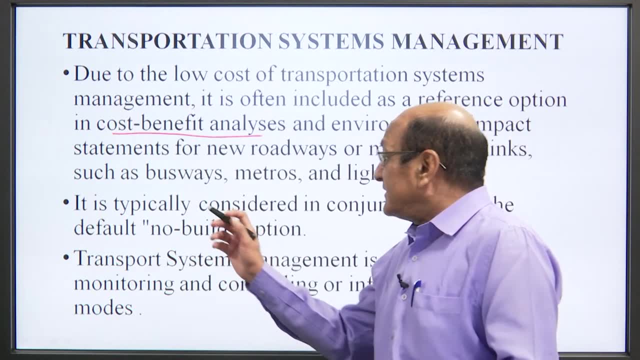 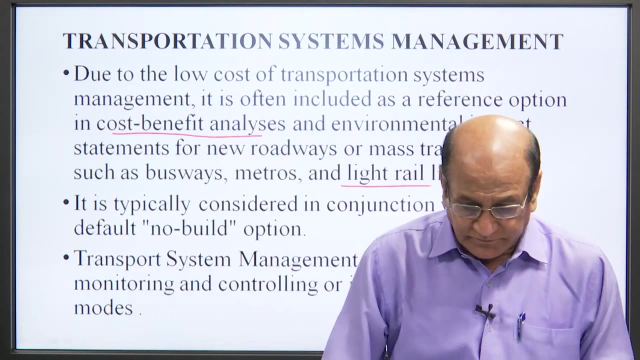 in cost and environmental impact statement, such as noise control, environmental impact statement or some other three types ofmm, for instance, and tailoring ok, braking system management. At least how many other properties are being done? These two are known: urban, busway, metros, light rail lines. It is typically considered in conjunction with the default. 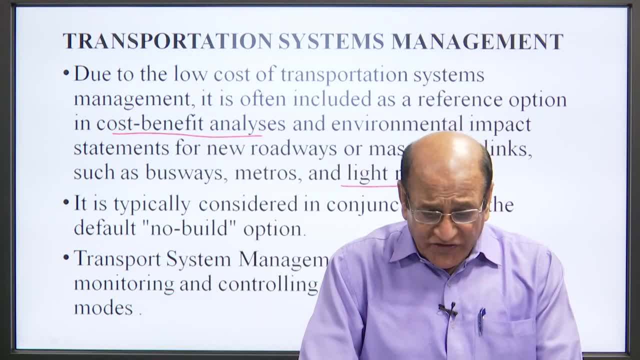 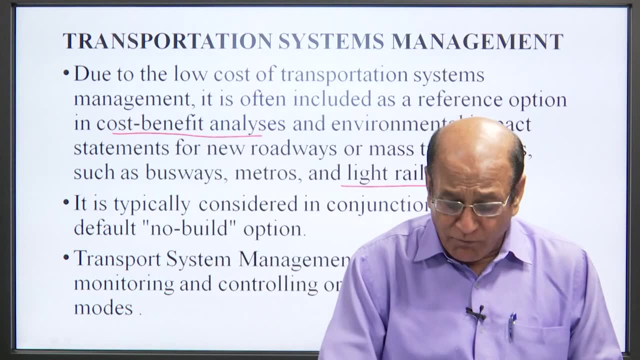 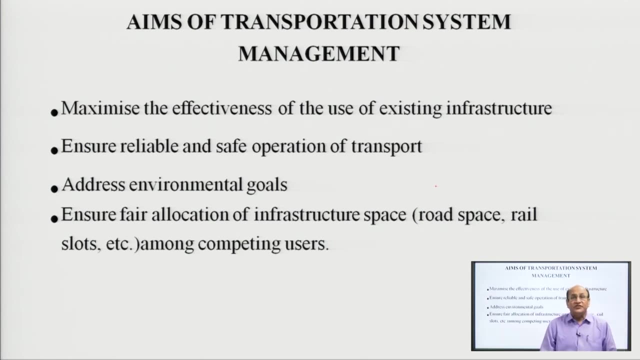 no built option. Transportation system management is a planning, monitoring and controlling or influencing of traffic modes. Now aim of transportation system management: Maximize the effectiveness of the use of existing infrastructure. Ensure reliable and safe operation of transport. Address environmental goal. 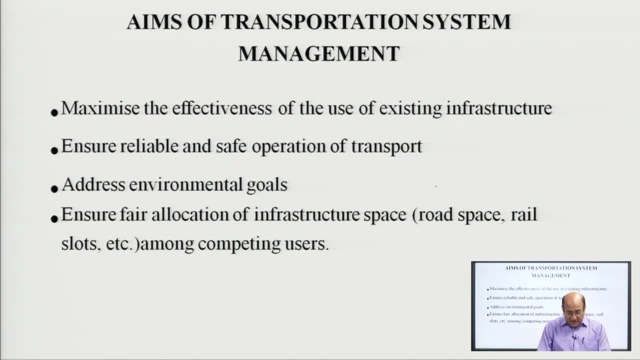 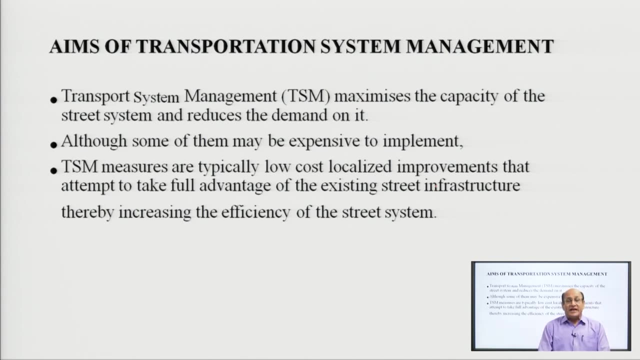 Ensure fair, English어주한 allocation of infrastructure space- road space, rail space, air slot, etc. among competing users. The transportation system management- we will say TSM- maximize the capacity of the street system and reduce the demand on it. Although some of them may be expensive to implement, TSM measures are typically low. 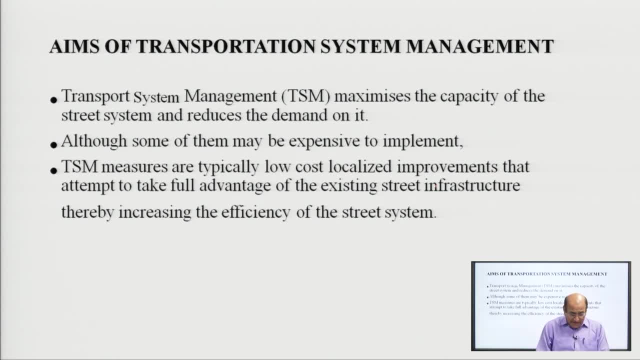 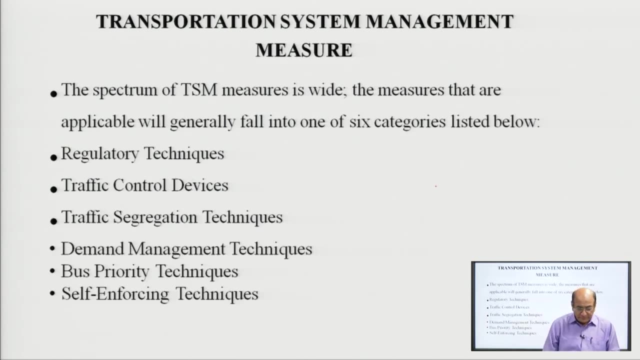 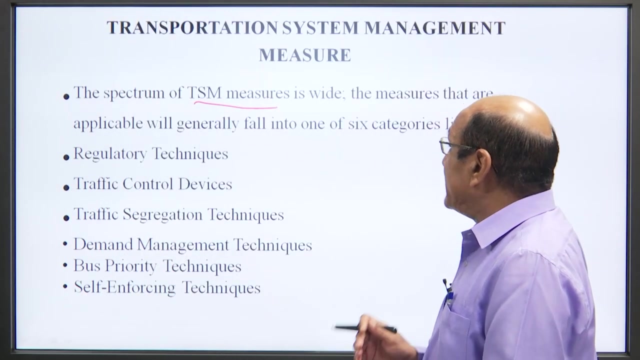 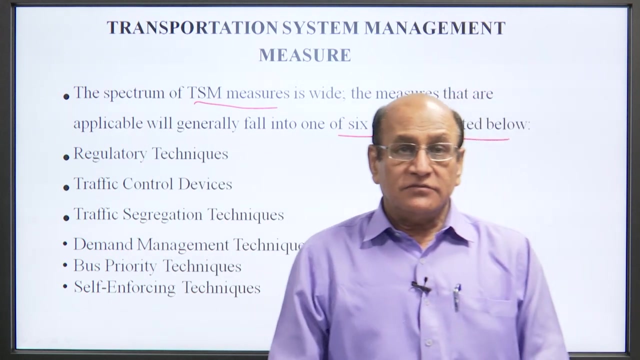 cost localized improvement that attempt to take full advantage of existing street infrastructure, thereby increasing the efficiency of the street system. Now, transportation system management measures. the spectrum of TSM measures is wide. The measures that are applicable will generally fall into one of the 6 categories listed below. 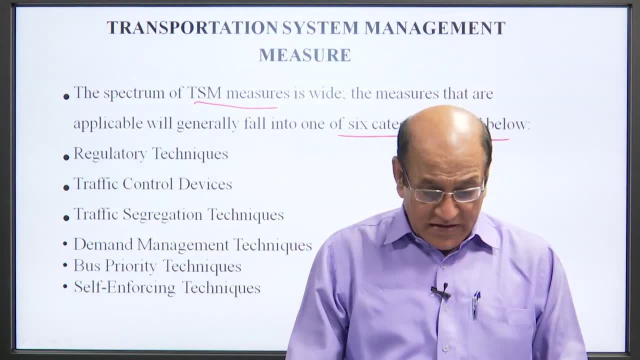 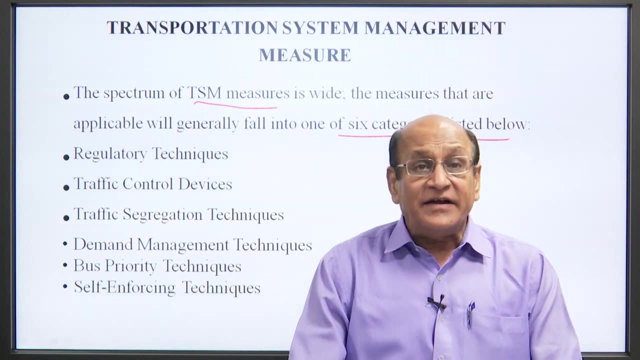 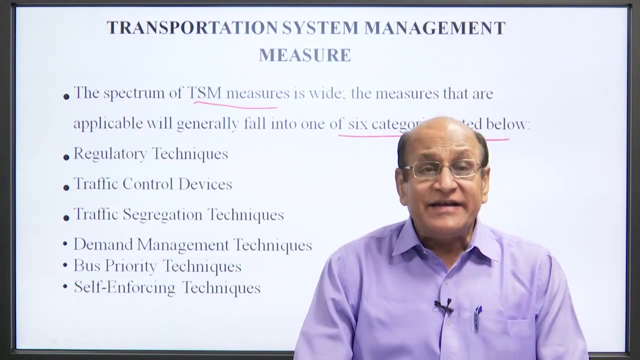 That are regulatory technique traffic control devices, Now transportation system management measures. The spectrum of TSM measures is wide. The measures that are applicable will generally fall into one of the 6 categories listed below: Traffic segregation technique, demand management technique, bus priority technique, self enforcing. 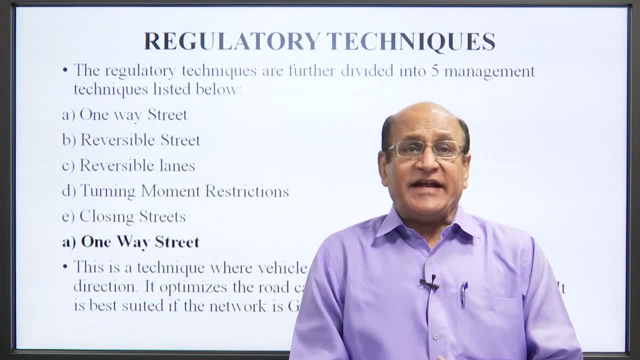 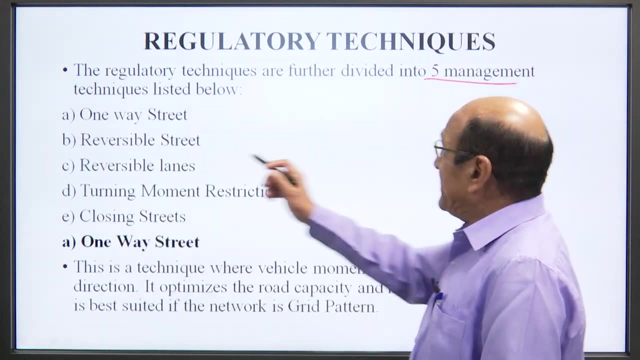 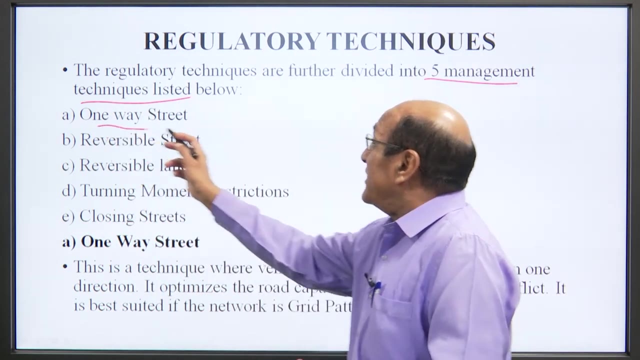 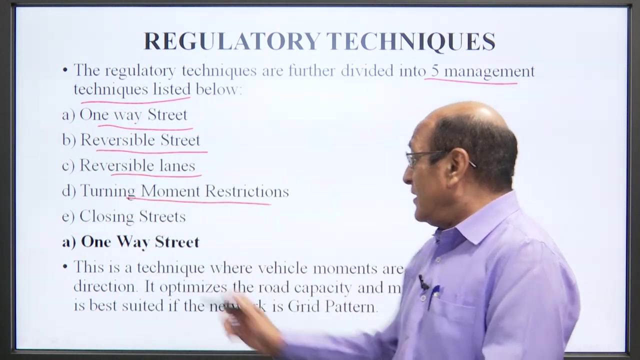 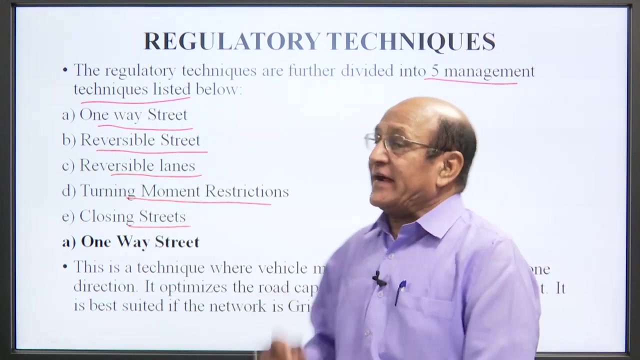 technique, regulatory technique. The regulatory technique are further divided into 5 management technique. What are they are? First is one way street, Reversible street, reversible lanes, Turning movement restriction, closing a street. So all five management techniques. First one is one way street. 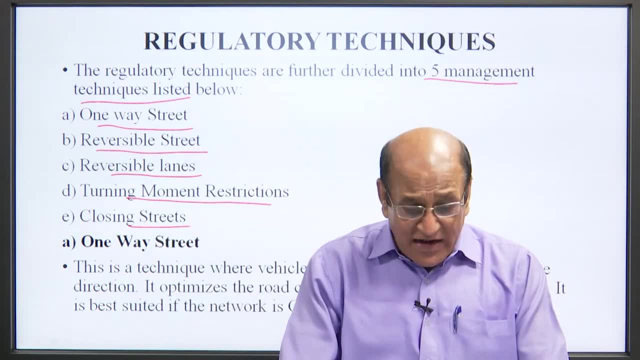 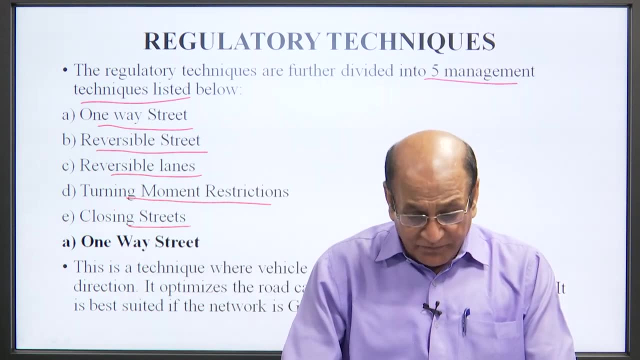 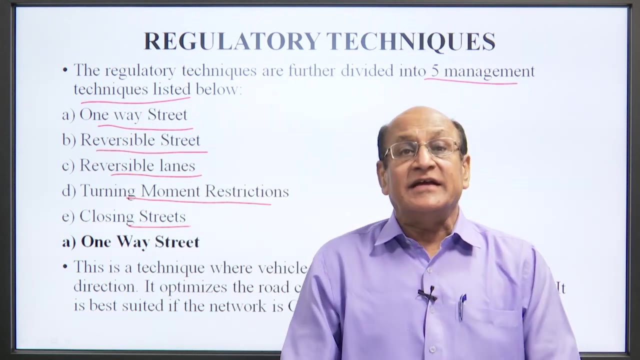 This is the technique where the vehicle moments are possible only in one direction. It optimizes the mobility to such aasi. It optimizes the mobility. Finally, the transverse invisibleorama Road capacity and minimize the conflict. It is the best suited if the network is in grid pattern. 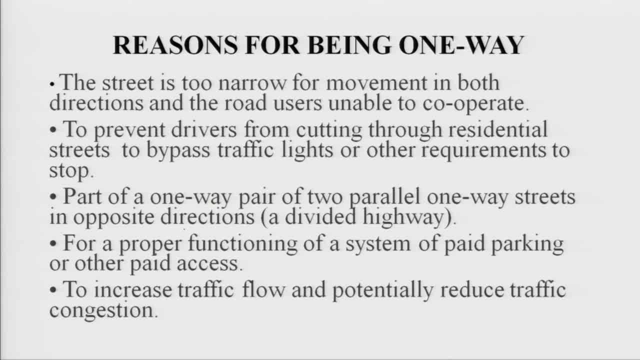 Reason for being one way: the street is too narrow for the moment in both direction and the road user unable to cooperate. Second, to prevent driver from cutting through residential street to bypass traffic light or other requirement to stop part of a one way pair of two parallel one way street in. 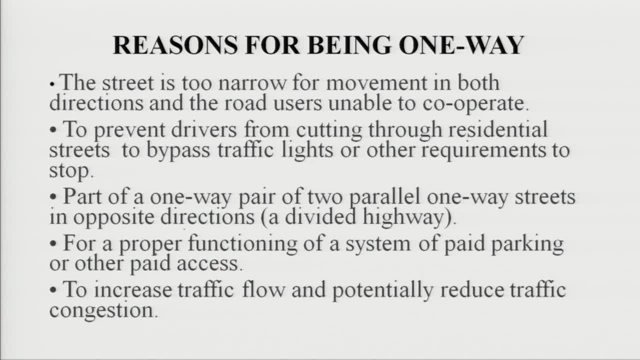 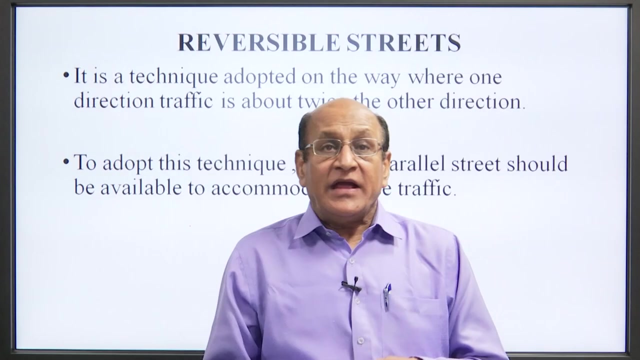 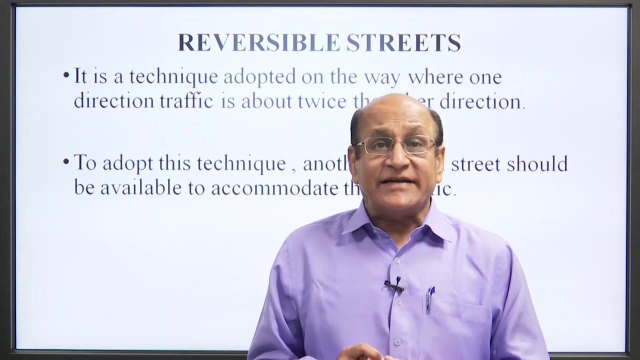 opposite direction. a divided highway For a proper functioning of a system, For a proper functioning of a system of paid parking or other paid access to increase traffic flow and potentially reduce the traffic congestion. Now, reversible street: it is a technique adopted on the way where one direction traffic is. 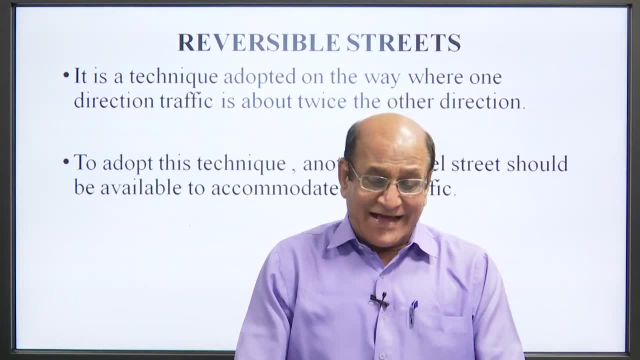 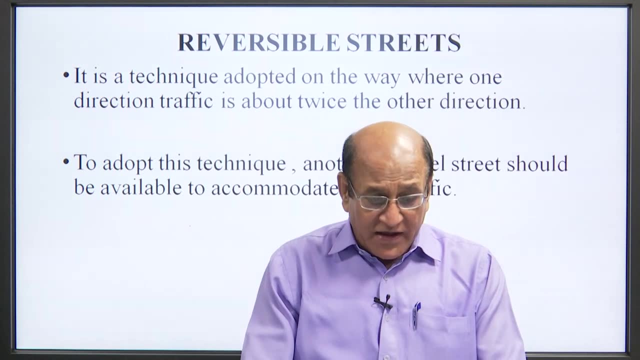 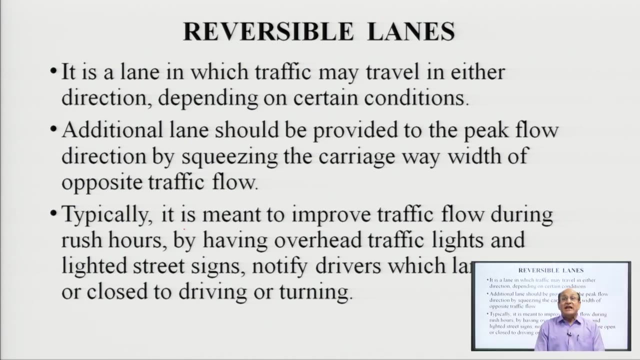 about twice the other direction, Now reversible street. it is a technique adopted on the way where one direction traffic is about twice the other direction. To adopt this technique, another parallel street should be available to accommodate those traffic Reverseable lanes. it is a lane in which traffic may be travel in either direction, depending 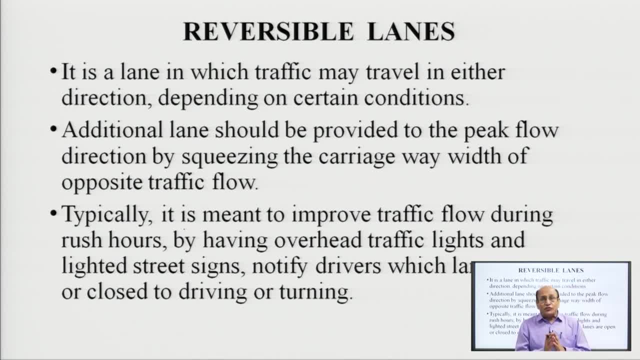 on a certain conditions. Additional lanes should be provided to the peak flow direction by a squinting the carriageway width of the lane. This is the opposite traffic flow. typically it is meant to improve traffic flow during rush hour by having overhead traffic light and lighted street sign. notify drivers which. 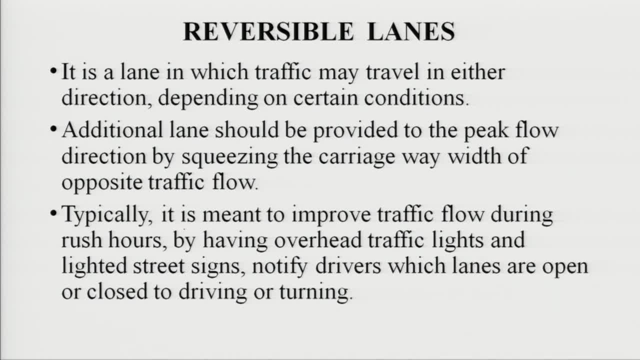 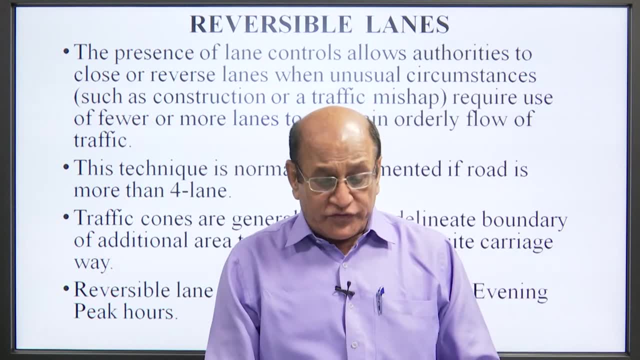 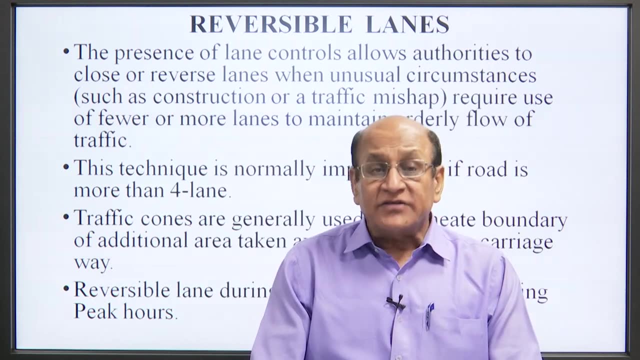 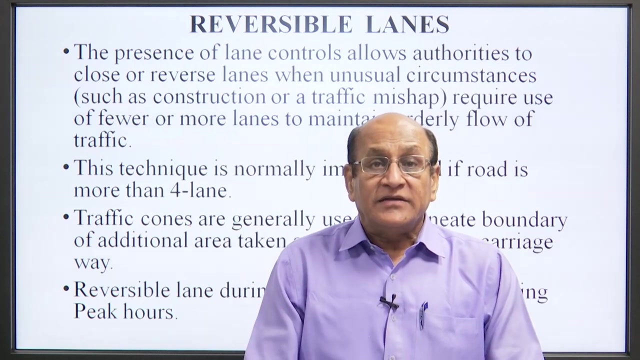 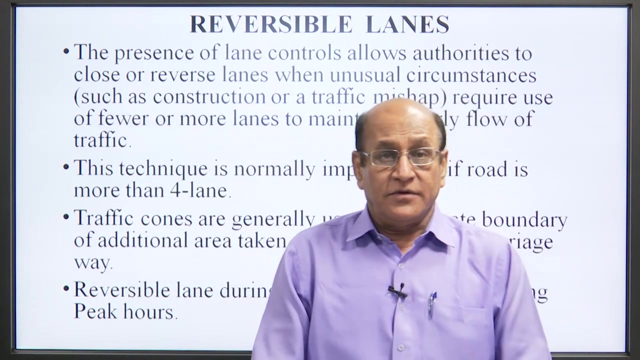 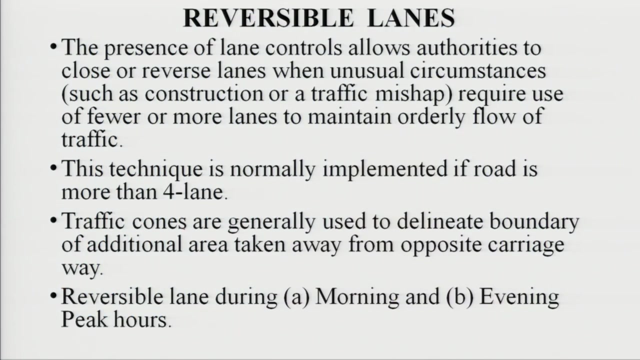 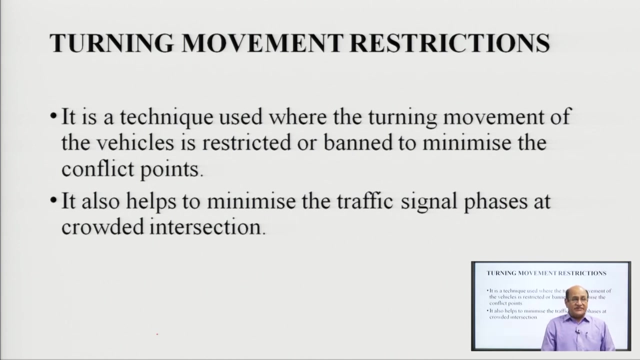 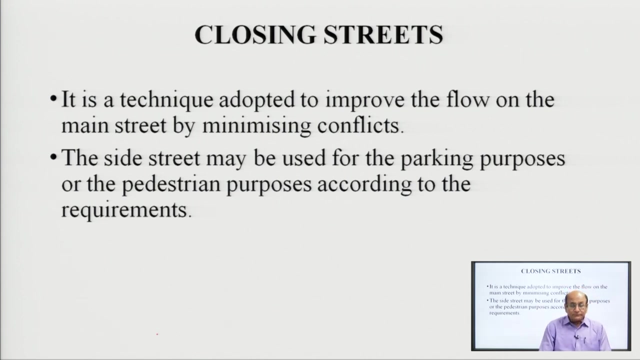 lane are open or closed by driving or turning, used when the turning moment of the vehicle is restricted or banned to minimize the conflict point. It also helps to minimize the traffic signal phases at crowded intersection. Closing a street: It is a technique adopted to improve the flow on the main street by minimizing 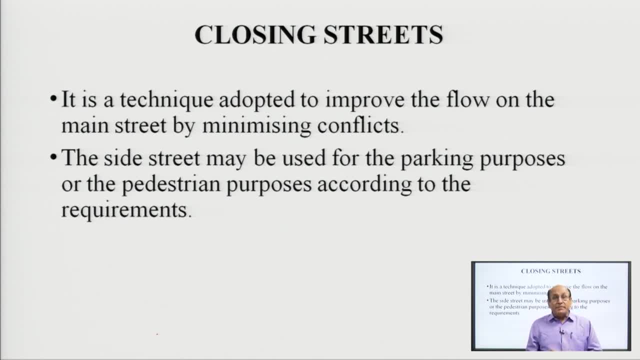 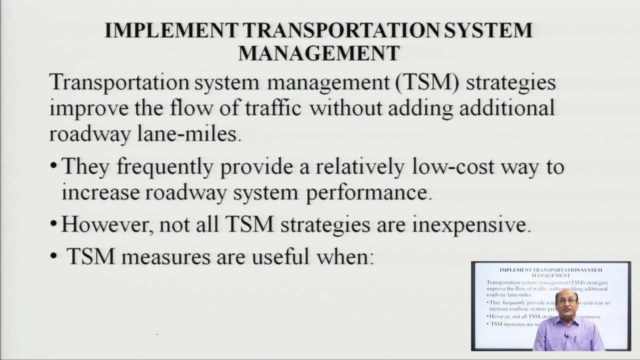 conflict. The side street may be used for the parking purposes or the pedestrian purposes, according to the requirement Implementation. transportation system management. Transportation system management strategy: improve the flow of traffic without adding additional roadway lanes. They frequently provide a relatively low cost way to increase roadway system performance. However, 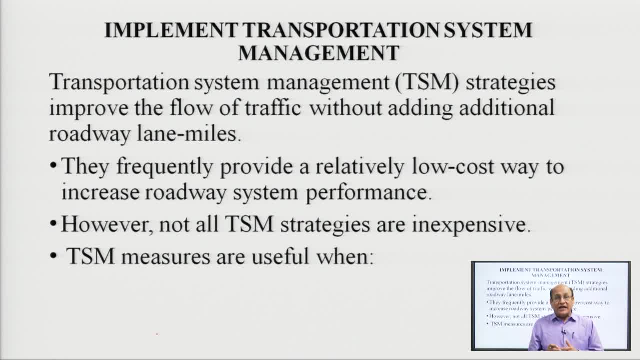 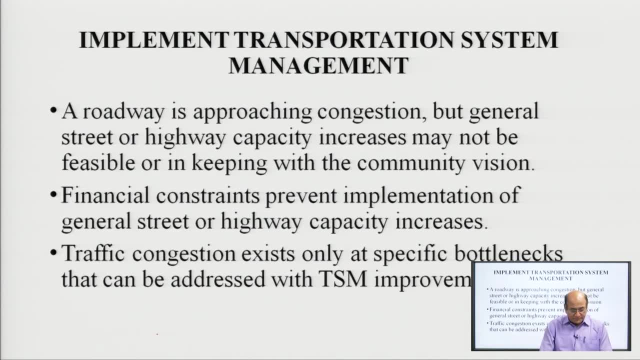 not all TSM strategy are inexpensive. TSM measures are useful when a roadway is approaching congestion, But general street or highway capacity increases may not be feasible or in keeping with the community vision. Financial constraint prevents implementation of a general street or highway capacity increases. 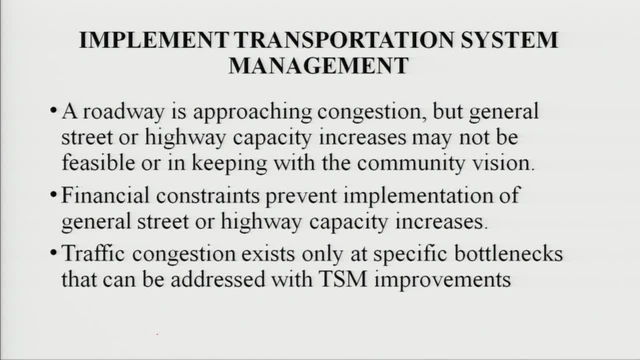 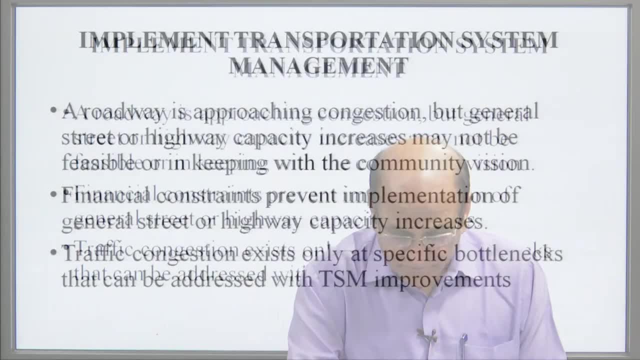 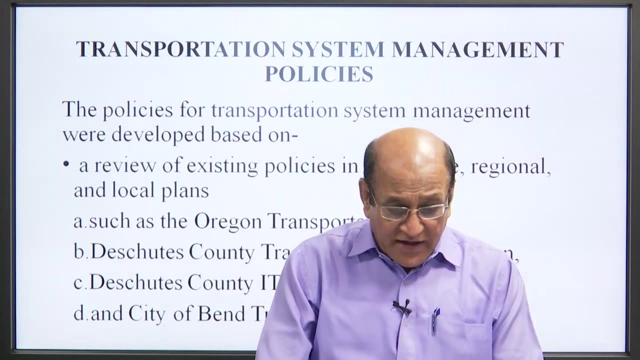 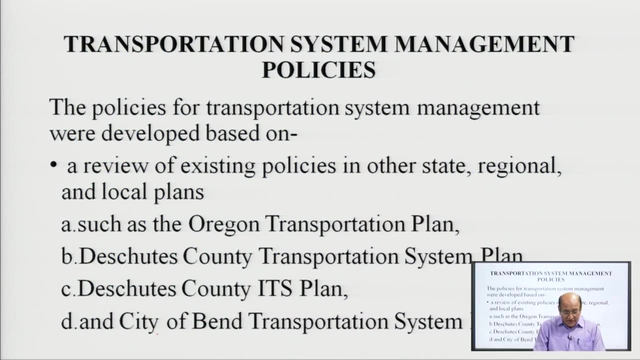 The traffic congestion exists only at the specific bottleneck. that can be addressed with TSM improvement. The policies for transportation system management were developed based on a review of existing policies in order. other state, regional or local plans, such as… CONSERVATIVE HIGH SCHOOL framework. 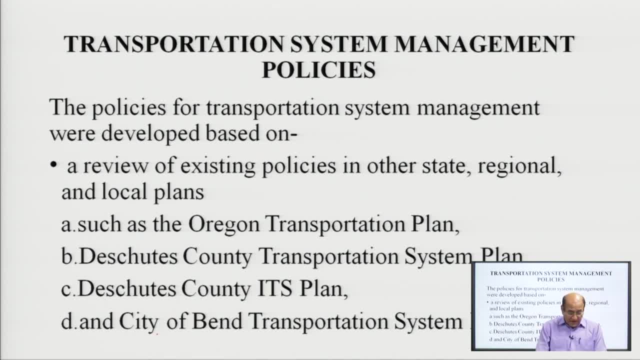 ан. Oregon Transportation Plan: Cost per Alma D ide. Bettica Auch 시 P acknowledgotte 험, vagie, absurde Low ContTEOS in traton, overland elementary and posthel. Austin City, Cade ITS plan and city of band transportation system plan. these are the plans, because these are. 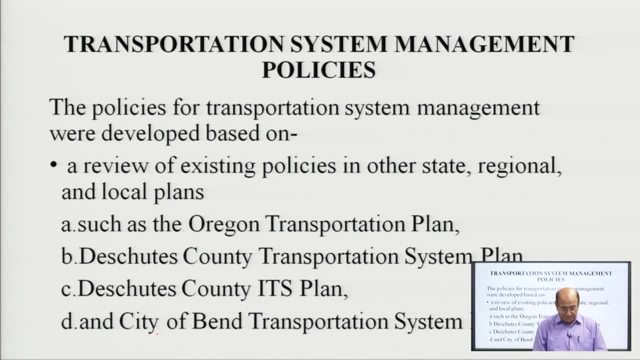 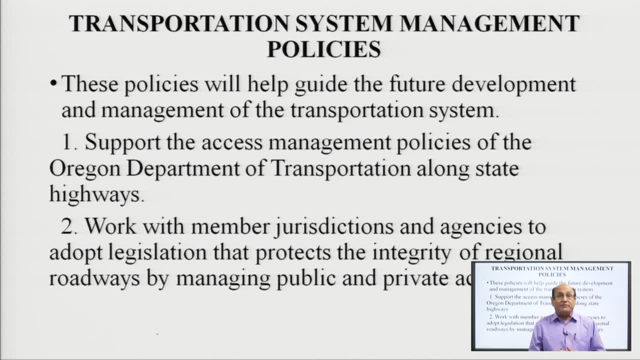 in a states a different type of transportation plans. These policies will help guide the future development and management of the transportation system. support the access management policies of the Oregon Department of Transportation along the state highway. work with the member jurisdiction and the agency to adopt legislation. 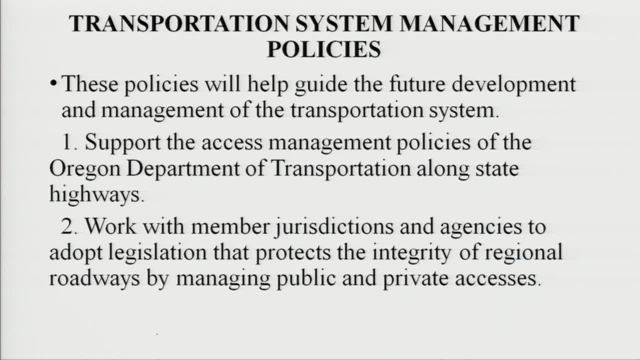 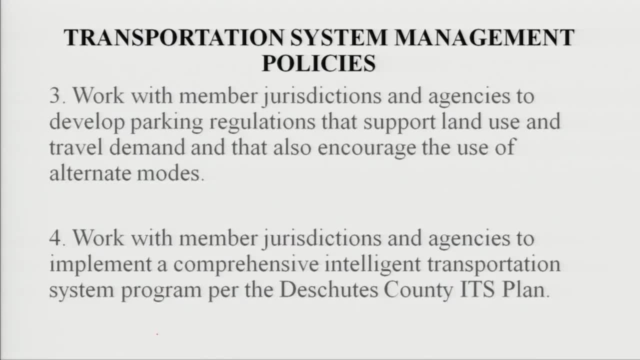 that protects the integrity of the regional roadway by managing public and a private road accesses. work with the member jurisdictions and agency to develop a parking regulation that support land use and travel demand and that also encourage the use of alternate modes. work with the member jurisdiction and agency to implement the comprehensive intelligent 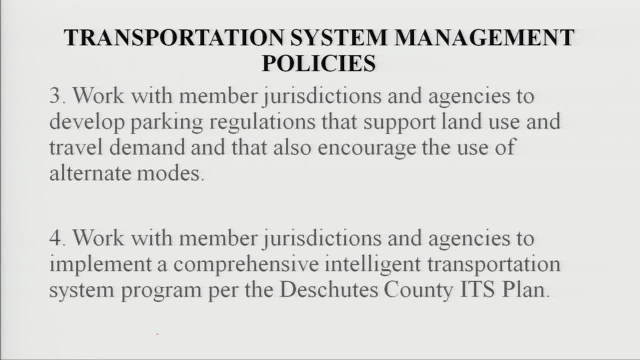 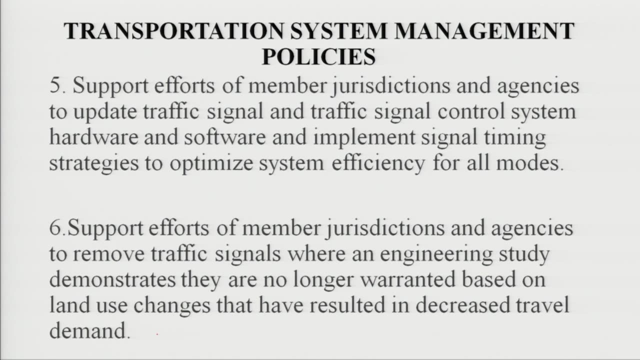 transportation system program. Okay Per the destitute country ITS plan. Support effort of the member jurisdiction and the agency to update traffic signal and traffic signal control system hardware and software and implement signaling timing strategy to optimize the system efficiency for all modes. Support efforts of the member jurisdiction and the agency to remove traffic signal by. 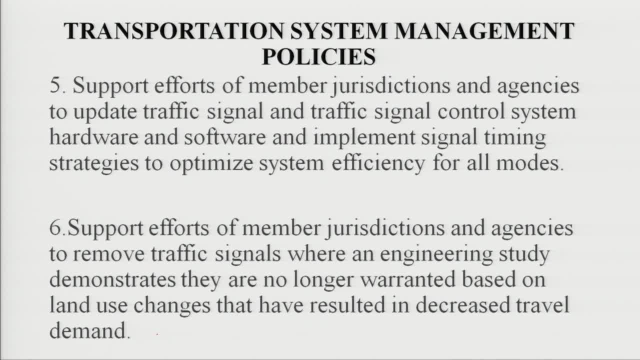 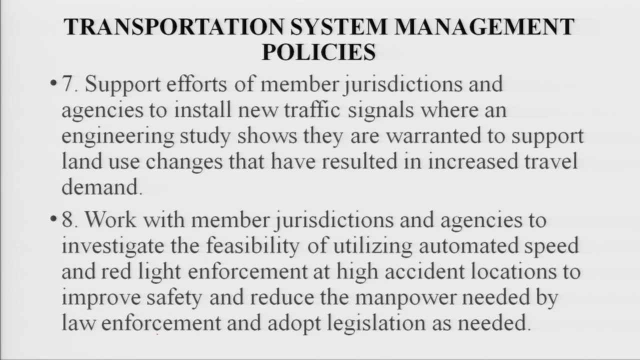 delivering greater ease of delivery to traffic, worry-free acres and injuries to vehicles and facilities To remove and eliminate traffic sickness from the roads and usages. The rest of the brown section works as the support effort of the member jurisdiction and the agency to remove traffic signal where an engineering, a study demonstrate they are no. 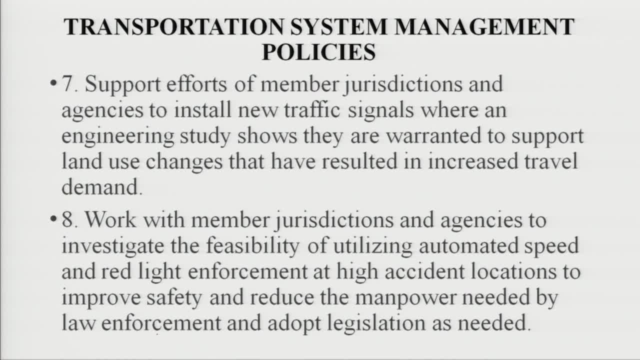 longer warranted based on land use charges that have resulted in decreased air travel demand. agency to install new traffic signal where an engineering study shows they are warranted to support the land use changes that have resulted in the increase the travel demand. Work with member jurisdiction and agency to investigate the feasibility of utilizing on. 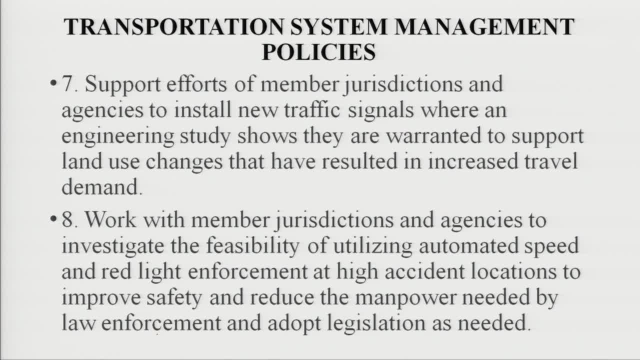 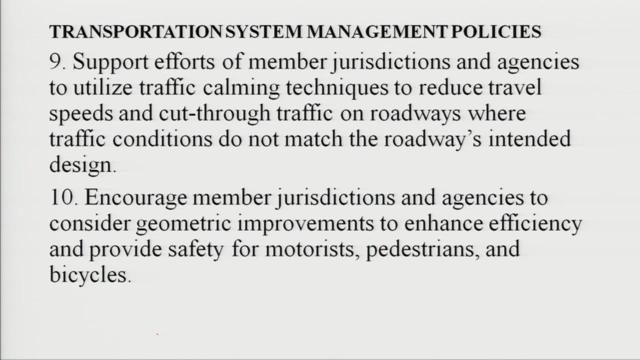 automated speed and red light enforcement at high accident location to improve safety and reduce the manpower needed by law enforcement and adopt legislation as needed. Support effort of member jurisdiction and agency to utilize traffic calming technique to reduce travel speed And cut Through traffic on roadways where the traffic condition do not match the roadway intended. 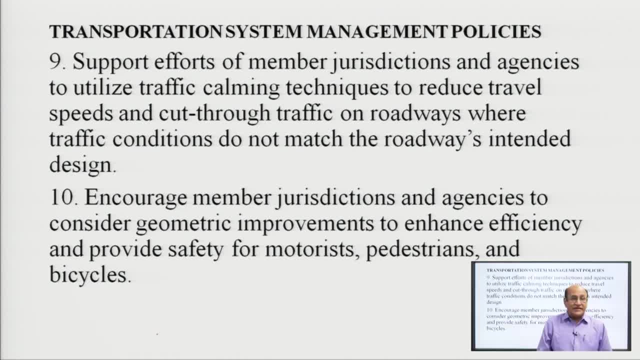 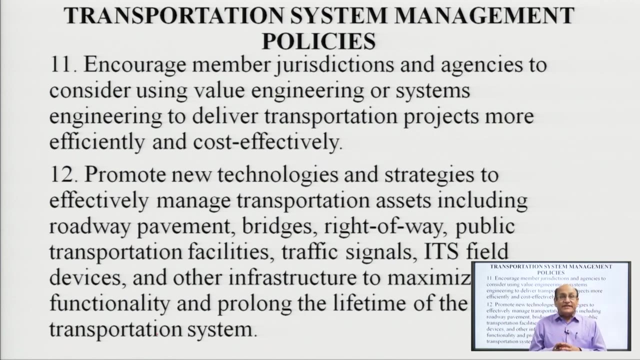 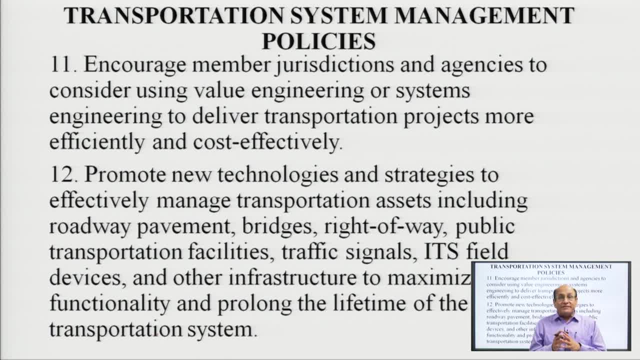 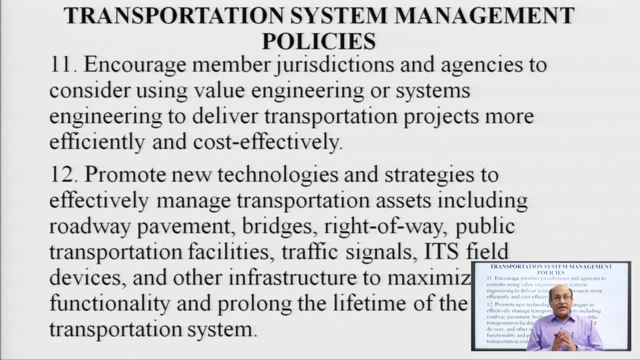 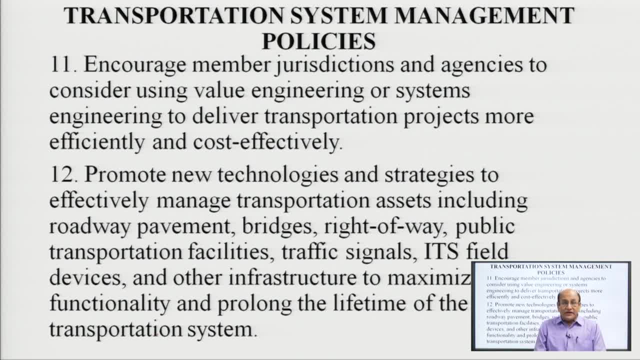 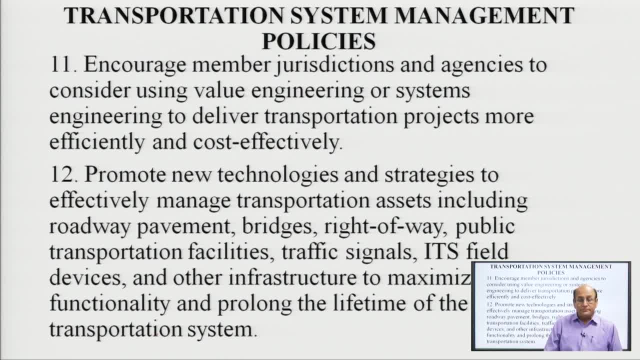 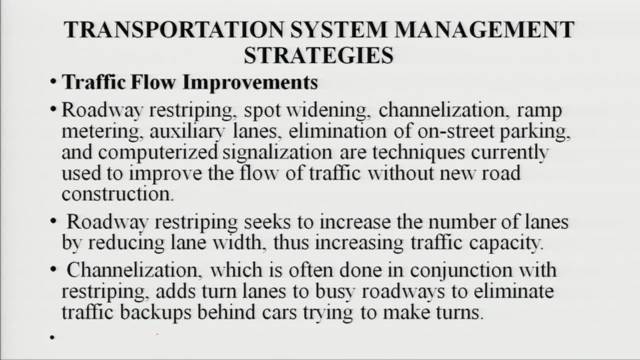 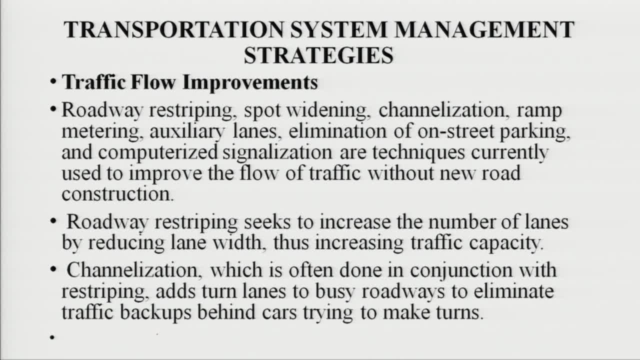 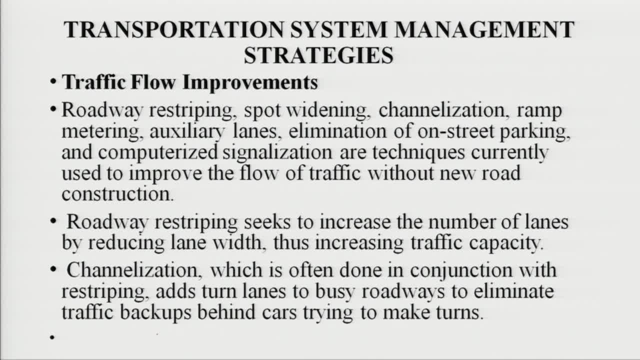 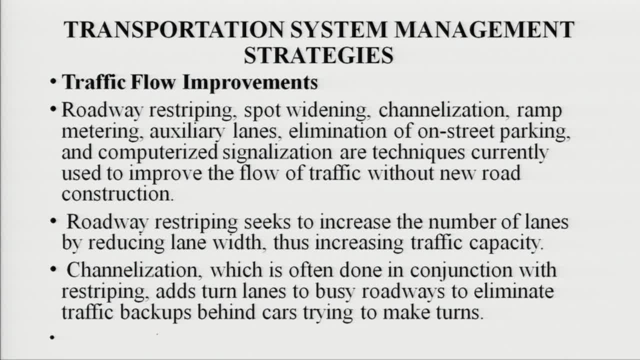 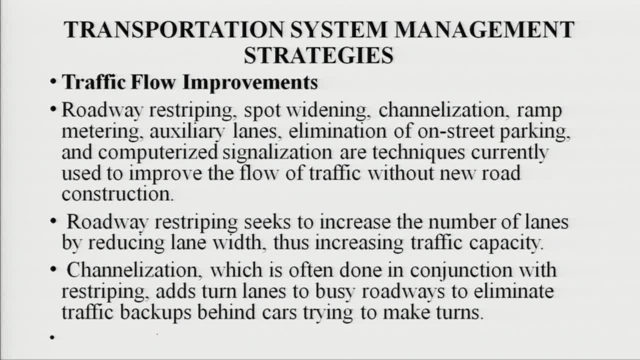 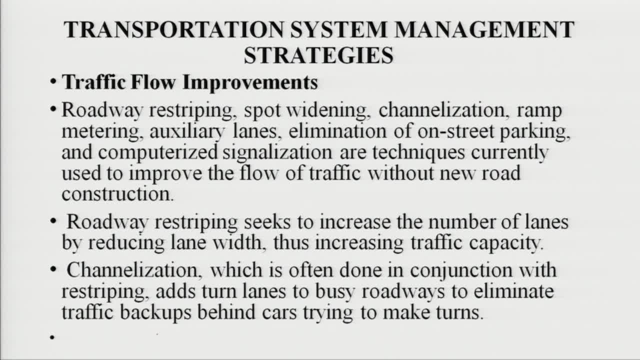 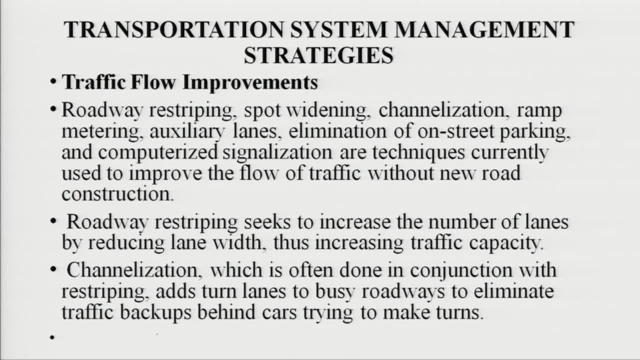 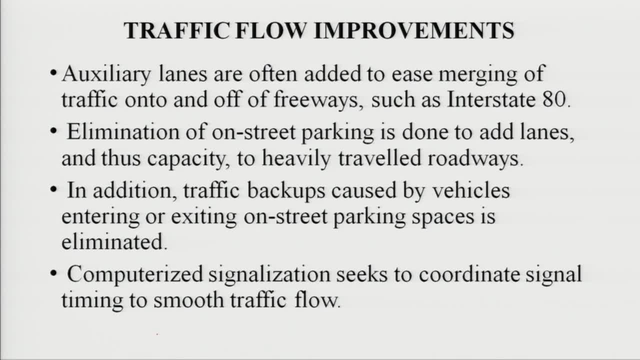 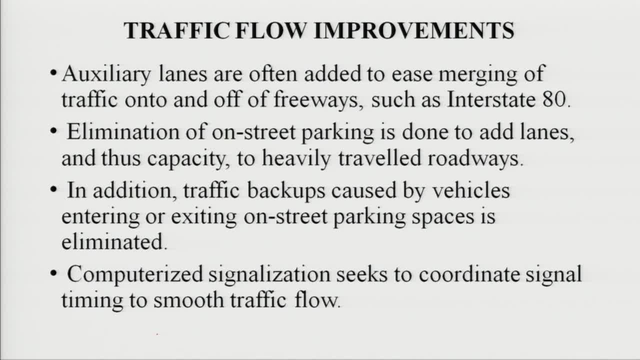 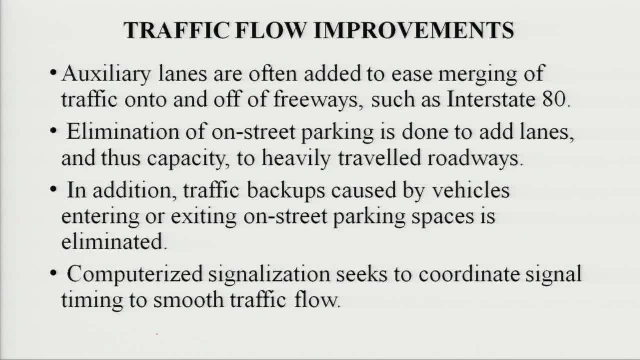 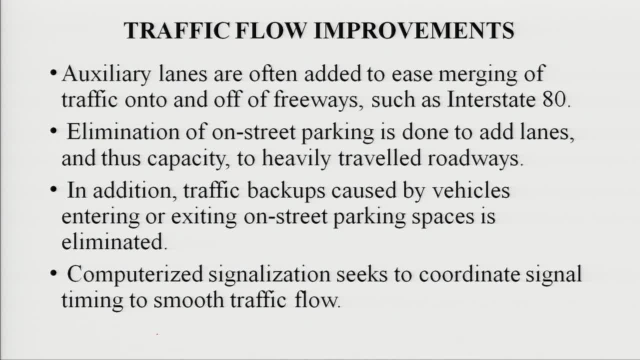 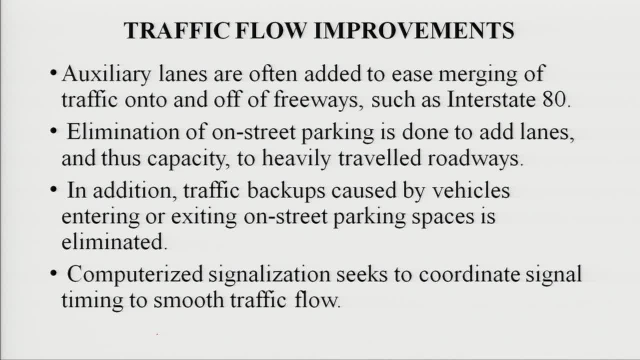 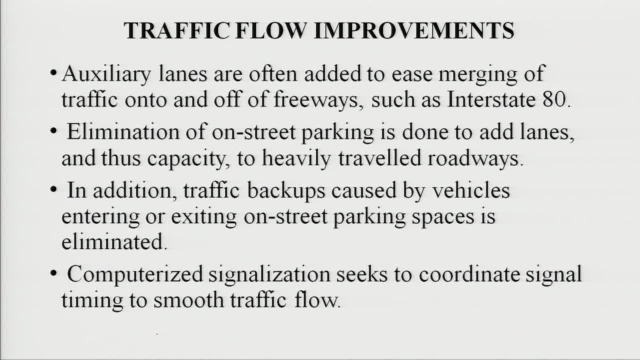 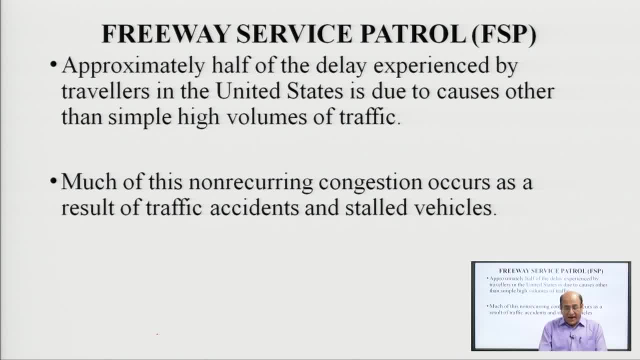 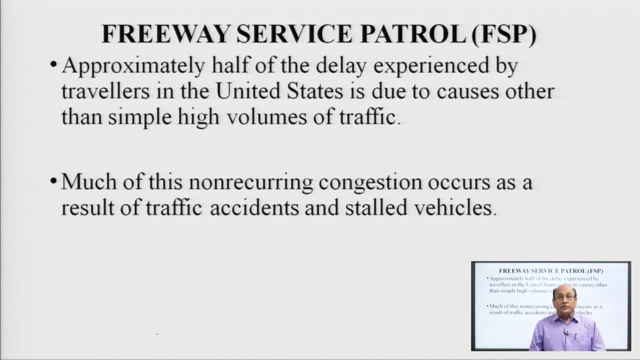 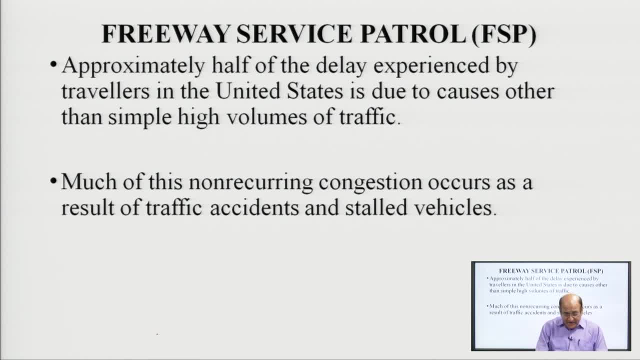 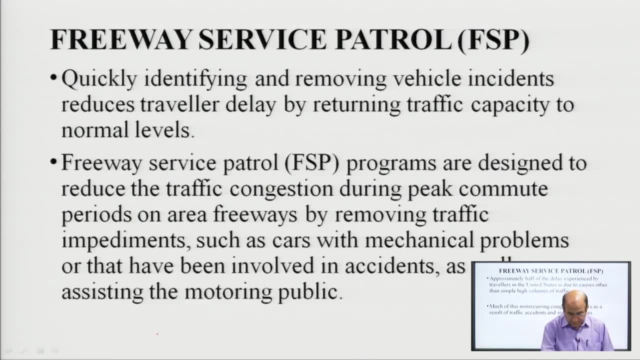 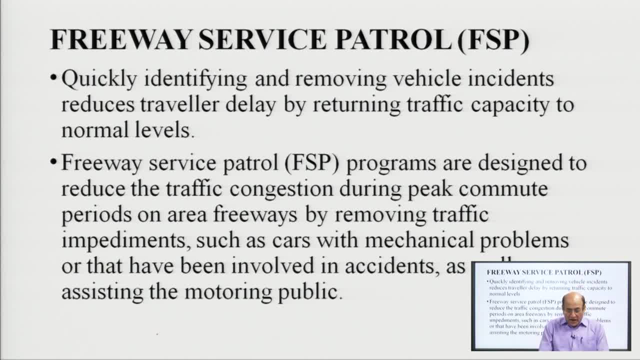 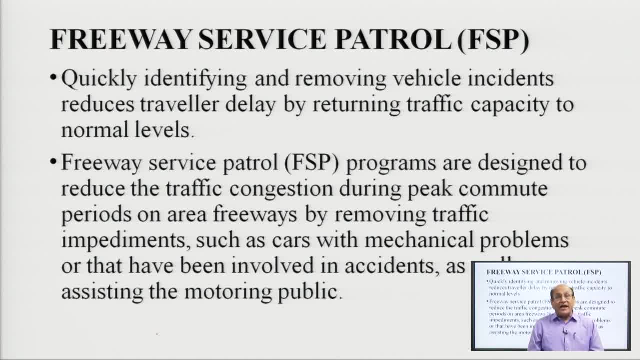 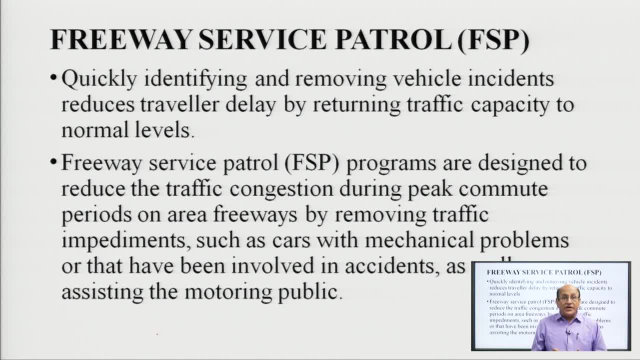 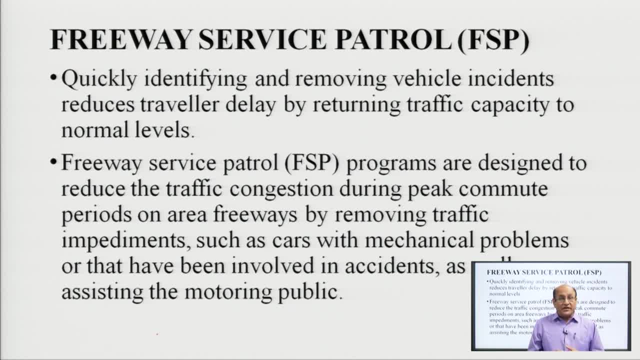 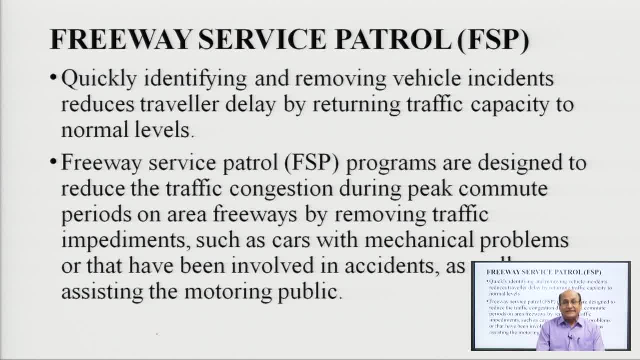 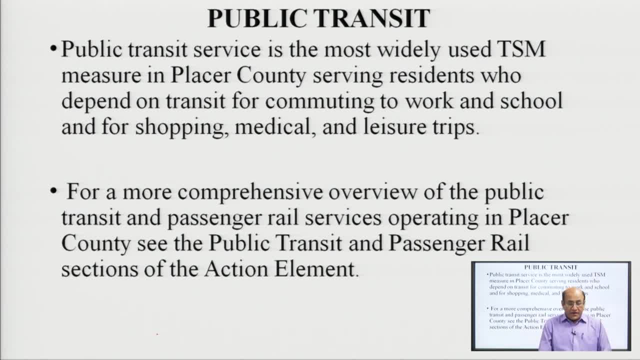 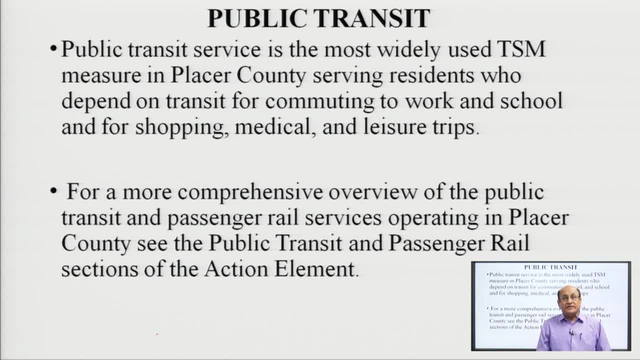 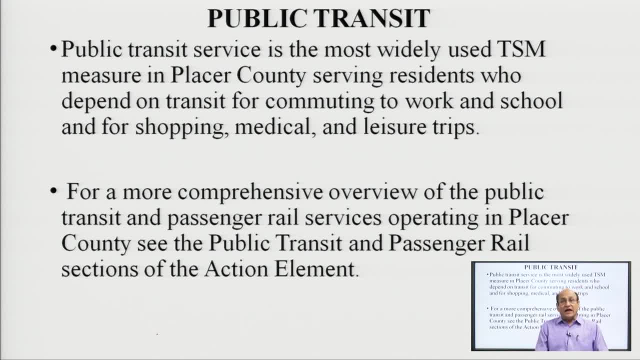 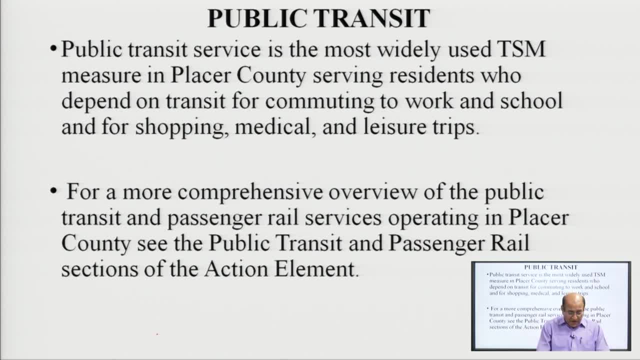 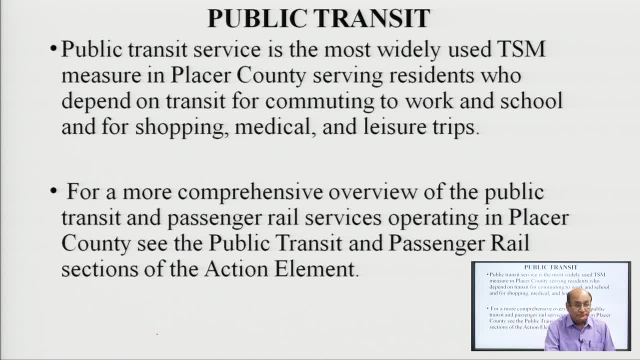 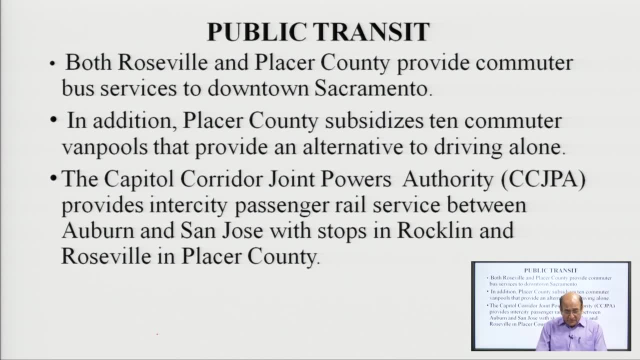 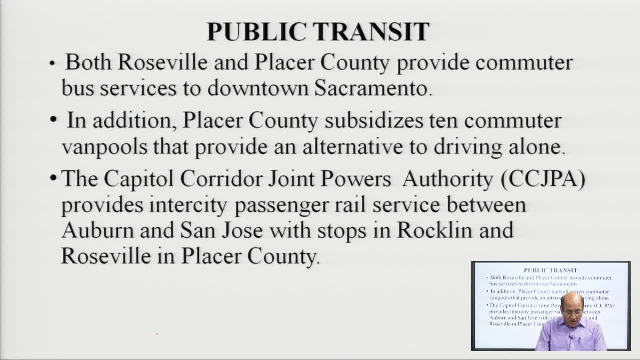 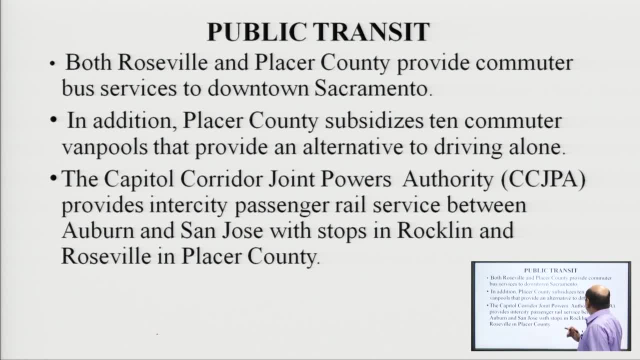 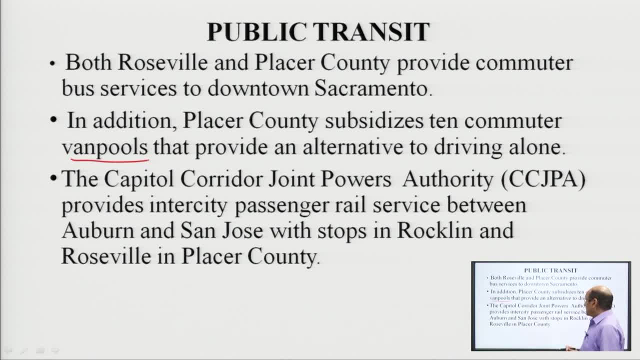 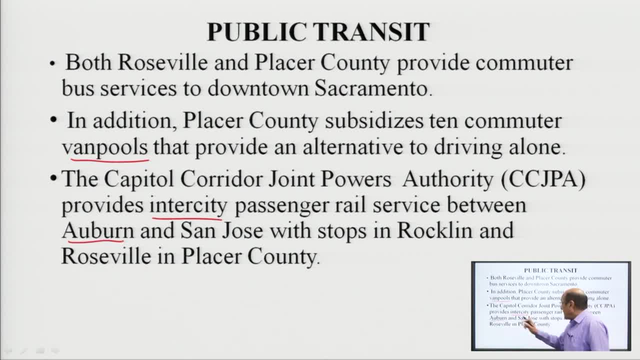 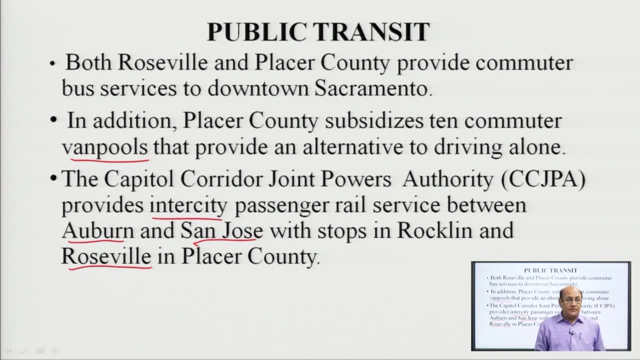 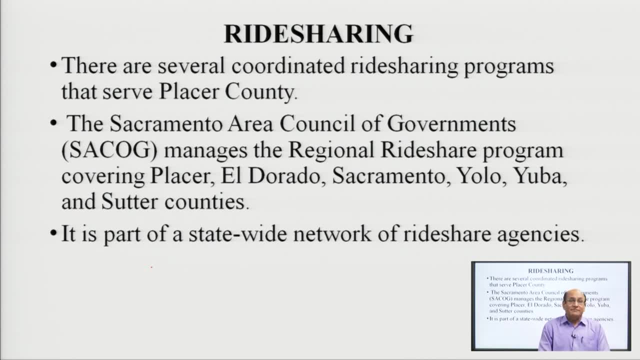 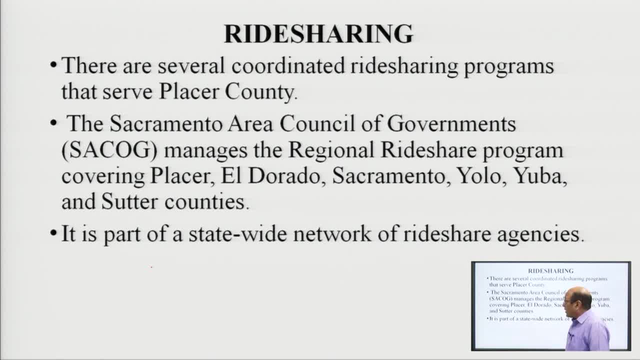 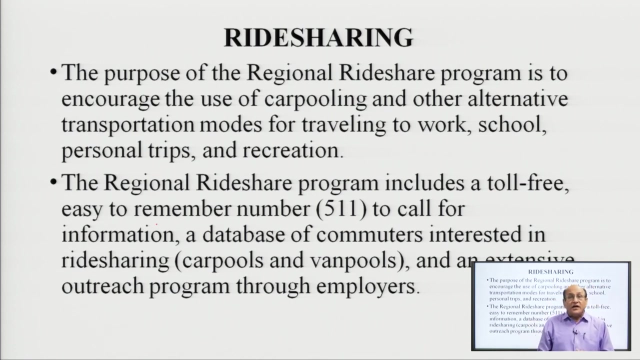 The Sacramento Area Council of Government manages the regional ride share program covering the placer E1,, Diado, Escarmento, Yellow, Yubo and Sutter countries. It is the part of a statewide network of the government. The purpose of the regional ride share program is to encourage the use of carpooling and 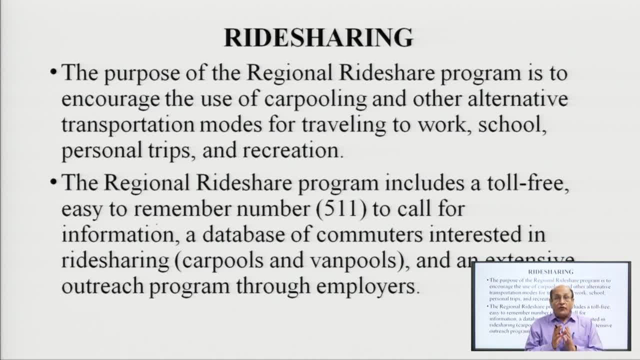 other alternative transportation mode for traveling to work, school, personal trips and recreation. The regional ride share program includes a total of 15,000 people. Number 3,, easy to remember, like 511, to call for the information and the data base of commuter. 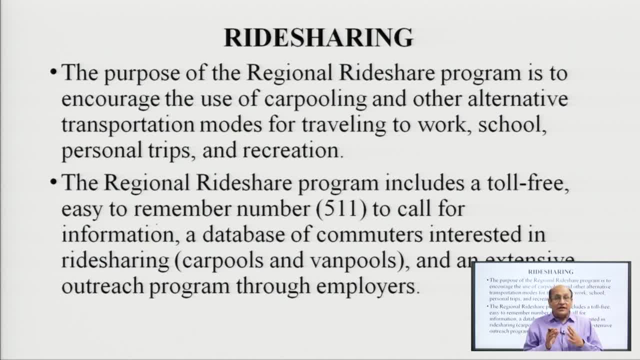 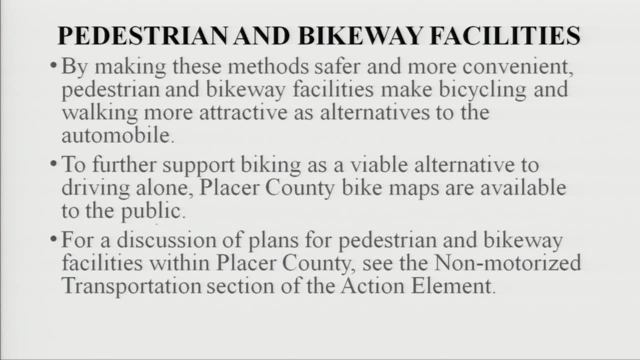 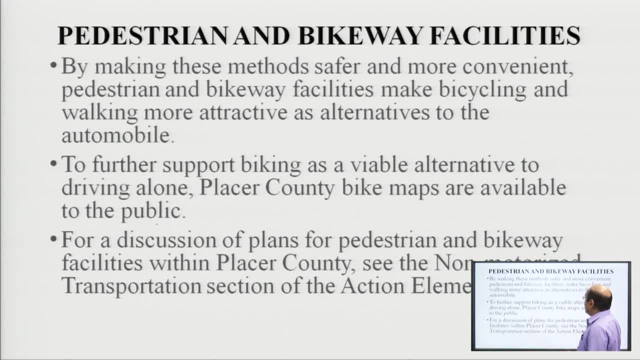 Pedestrian and bike way facilities, Making these methods safer and more convenient. Pedestrian and bike way facilities make the bicycle and walking more attractive than alternative to the automobile. to further support biking as an available alternative to driving alone. placer country COMMUTE or RIDE SERVICE program. 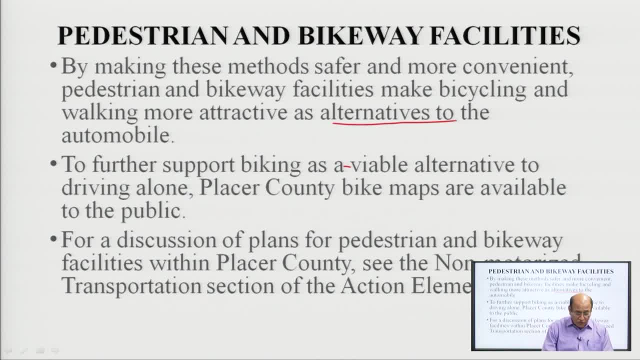 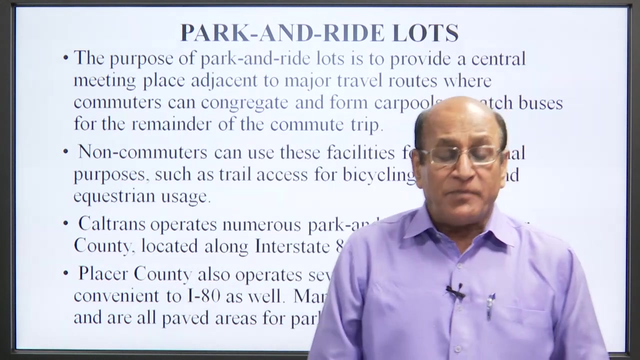 country. bike maps are available to the public for a discussion of a plan for pedestrian and bike way the facility with the pacer country: see the non-motorized transportation section of the action element park and ride lots. the purpose of the park and ride lots is provide: 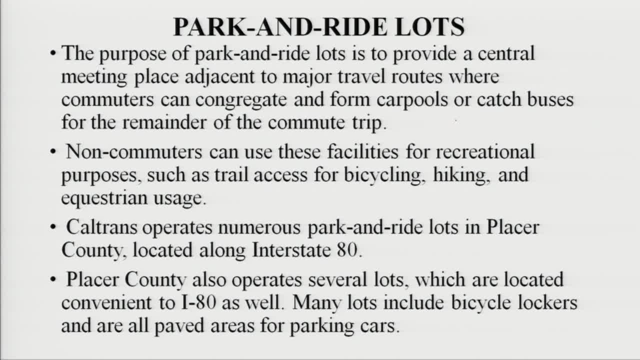 a central meeting place adjacent to the major travel route where the commuter can congregate and for carpool or catch buses for the reminder of the commute trip. non-commuter can use these facility for recreational purposes, such as rail across, for bicycling and for the commuter. 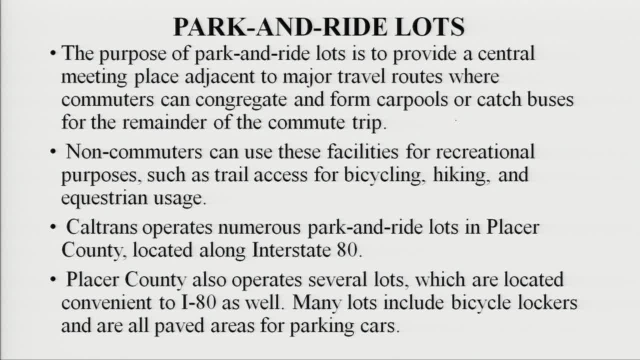 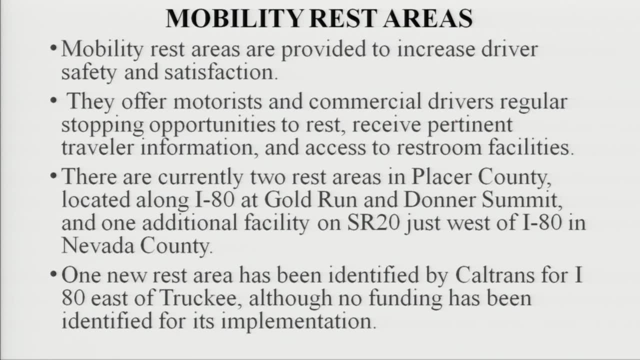 can take a loop car for both the back bike and the back ride and also the back ride and the back ride and in the back parking. there is a bicycle parking lot along the level road which is the best place to use this parking lot along the top of the park for each location. 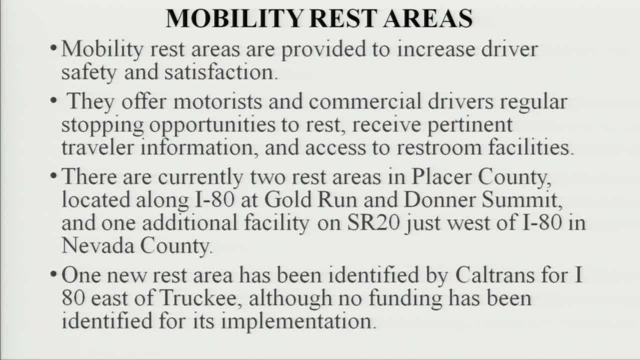 and the pacer park is also first on to the central route and the pacer to the south end of the park is the best spot to use this parking lot along the i-80 mobility rest area. mobility rest area are to provide to increase driver safety and satisfaction. they offer motorriding. 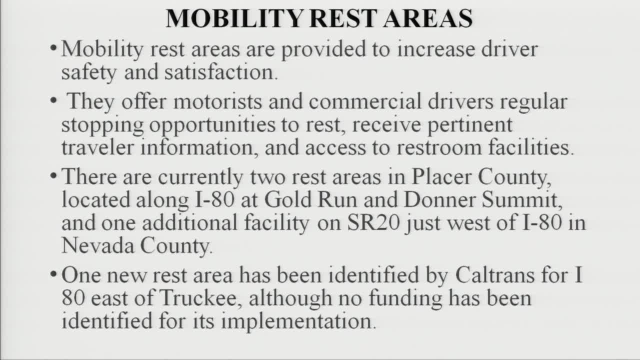 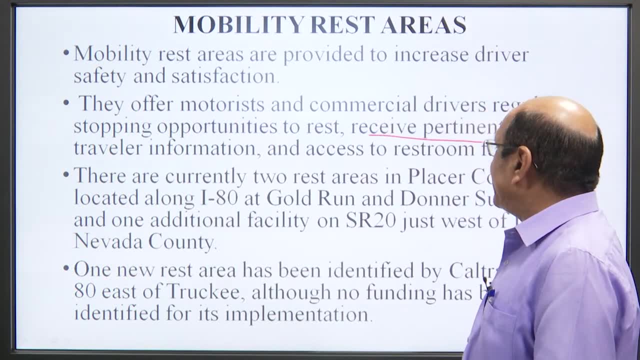 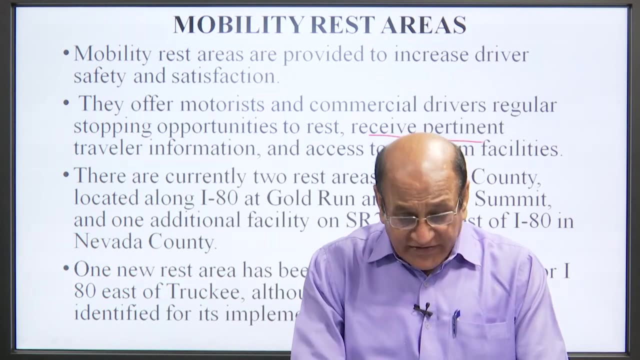 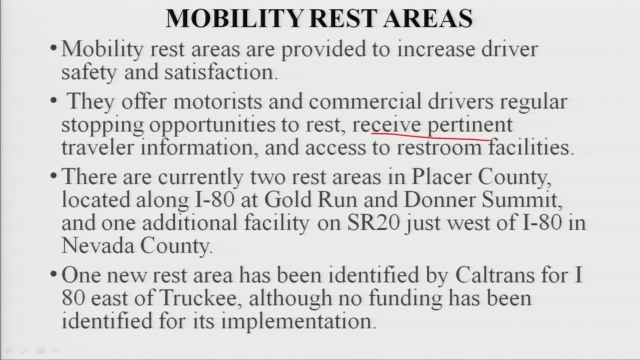 tourist and commercial drivers regularly stopping opportunities to rest, receive pertinent traveller's information and access to re-astrom facilities. There are currently two rest area in placer country located: I-80 at golden run and donor summit, and one additional facility at SR-20 just west of I-80 in Nevada country. 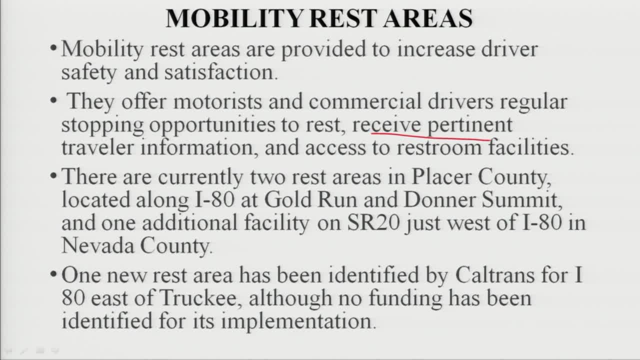 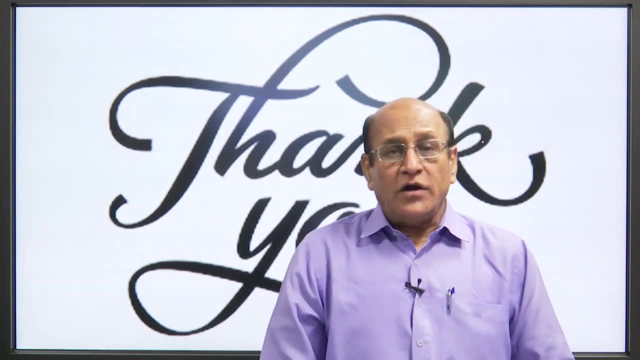 One new rest area has been identified by the Caltrans for I-80 east of Turkey, although no funding has been identified for its implementation. So this is the All about the traffic system management. thank you very much. thank you.